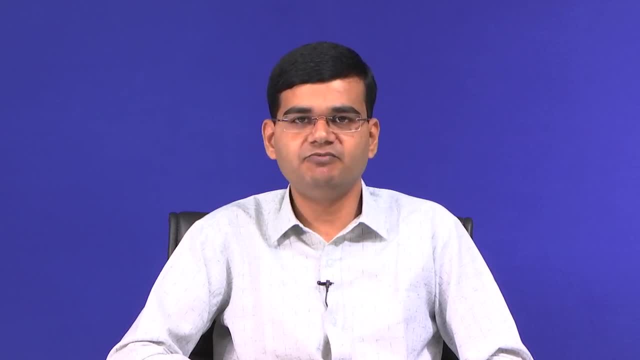 systems Which undergo change with time, and we would be studying such systems in this course. Now, to take a simple example, we can imagine that we enter a hot and humid room, which is say, at a temperature of 40 degree centigrade, and we want a comfortable environment and 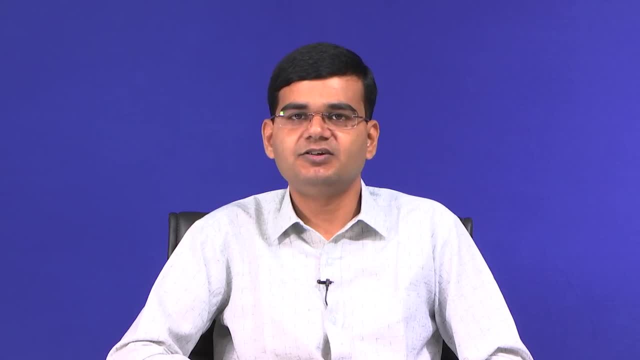 we want the temperature to be maintained at, say, 22 degree centigrade, Obviously, what we will do is Put an air conditioner which will control the temperature of the room. What we very often do not consider is that, apart from controlling the temperature of the room, there is something. 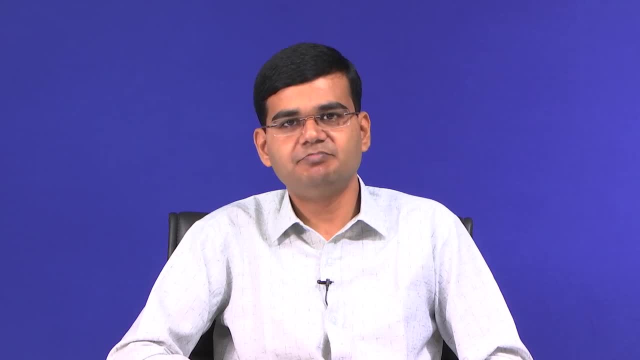 else, which is also going on As you enter the room. the temperature is at 40 degree centigrade and the temperature has to decrease to 22 degree centigrade, And after the temperature has been reached to 22 degree centigrade, it has to be maintained constant. So what? 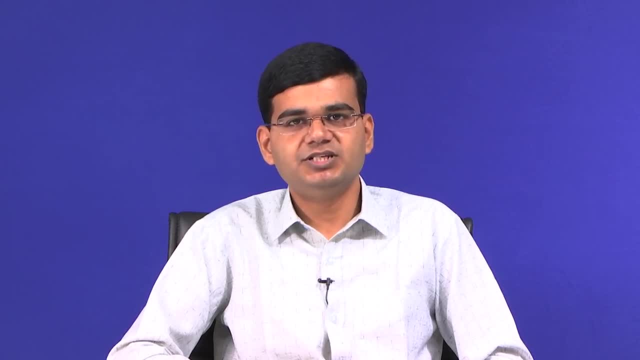 happens is that there is a period during which the temperature of the room changes, So therefore, this is a dynamical system. To take an example from industry, imagine that we have a petrochemical plant in which there is a fixed bed reactor And we want to maintain constant composition. 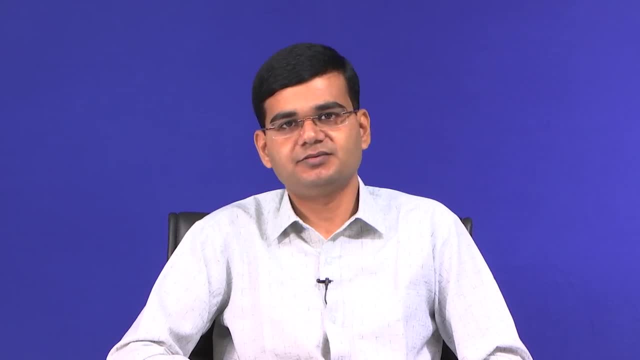 constant temperature, constant pressure inside the reactor. Since we know that packed bed reactors are typically operated at steady state, we would assume that there would be a control system which would be maintaining all the properties associated with the system as constants. But before this condition of constant properties, 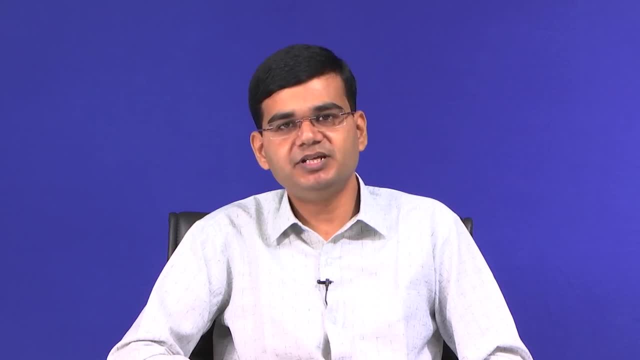 is reached, there would be a start up period during which the properties would change with time. Therefore, this is also an example of a dynamical system. So while during the early education of chemical engineering, the students are introduced to the concept of process dynamics, 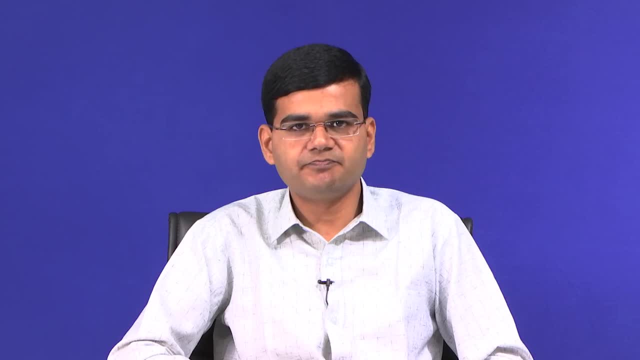 during courses like process instrumentation and control or process dynamics and control or chemical process control or simply control engineering. The real vastness of the domain of process dynamics is very often missed because the relevance is often taught with interest to process control. But we would realize during this course that process and process dynamics 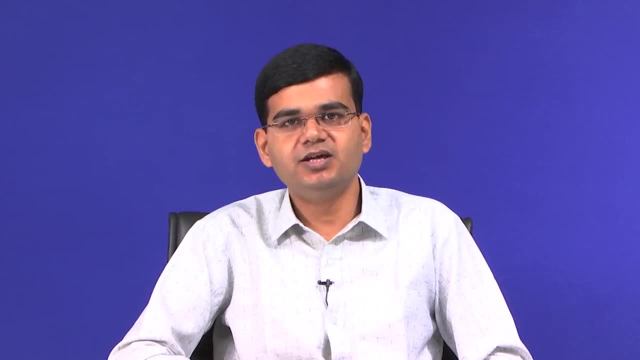 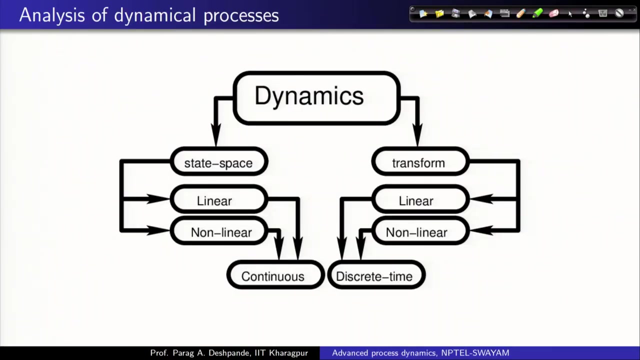 in itself is a standalone and a vast domain of process engineering which needs attention, and that is precisely what has been the intention behind developing this course. So, to analyze the dynamics of a system, We have basically two methods or two approaches: the one which is shown on the left hand side. 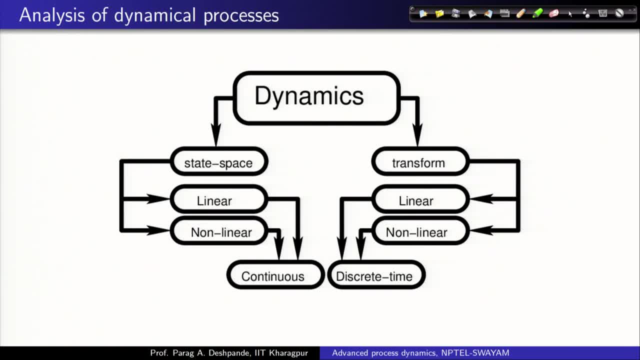 is the state space domain approach and the one on the right hand side is the transform domain approach. During the early stages of undergrad education you get introduced to the transform domain approach. However, a very generic and a vast approach is the state space domain analysis, in which one can understand all the possibilities of the system, which 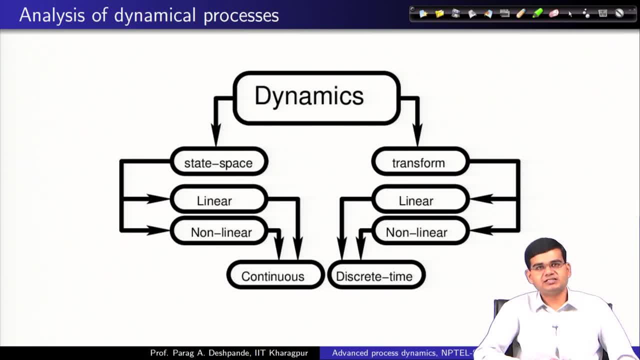 the system can sample, and we will initiate our discussion of this course by state space domain analysis and subsequently, towards the later part of the course, we will come to transform domain analysis. The systems that we typically study are linear systems, but in reality, majority of the systems are non-linear, So therefore we would take examples of non-linear systems. 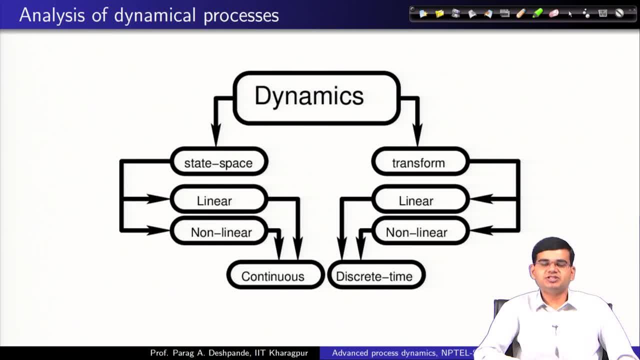 and see how approximations which are made for the study of linear systems do confirm to non-linear systems or where they deviate from the approximations. However, in all of these cases, linear system analysis makes a good case for as a starting point for the 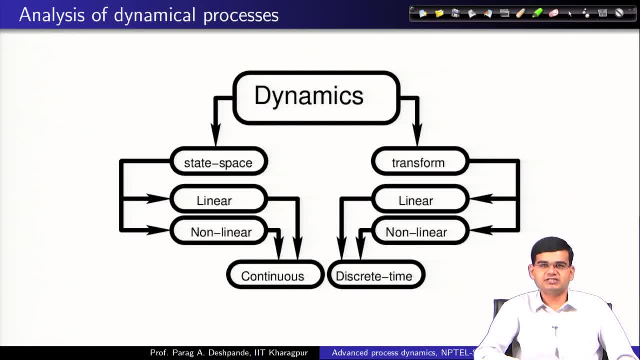 analysis of non-linear systems and therefore we will initiate our discussion with linear systems and we will subsequently graduate to more complex non-linear system analysis. The examples of temperature inside a room or temperature pressure, concentration, etcetera, inside a reactor were the examples where the system was operating in a continuous domain. 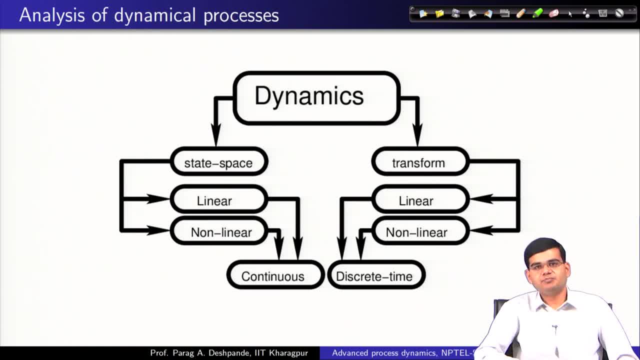 However, these days most of the process control is employed. So here we have to consider management and the sampling method for the analysis. So in this particular case we are going to look at the analysis of an instrument like we have the instrument called any other instrument, and this instrument is called the seeds. so 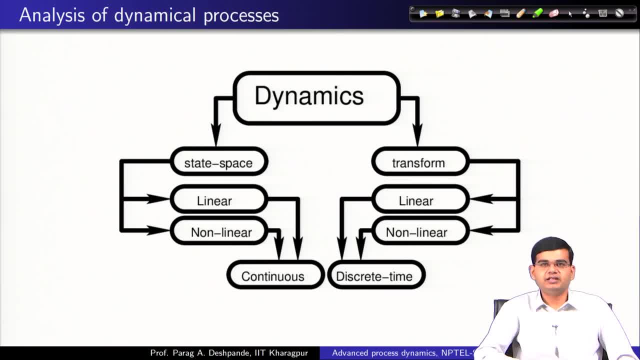 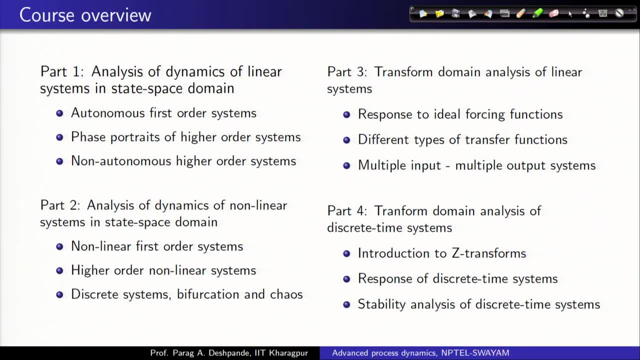 you need to be aware. if you decide to use the seeds or not to use the seeds, you have to be aware of the seeds and so all the steps we need to cover. So, in this particular case, we are going to have a non-linear analysis, but we have the 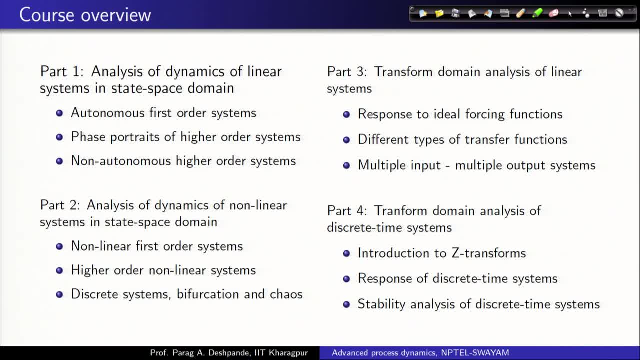 analysis of the in the next part. So we need to verify the analysis of the instrument systems in state space domain. After understanding the linear systems, we will go to the state space domain analysis of non-linear systems And then we will do the analysis of linear. 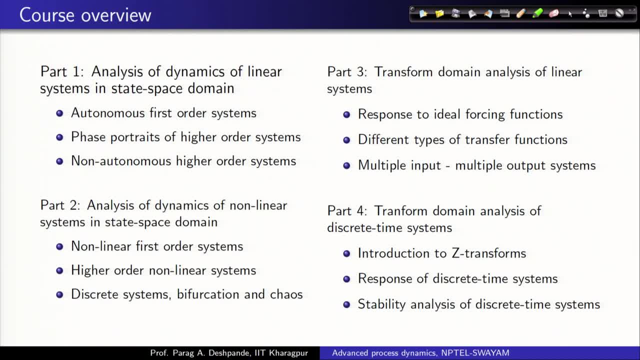 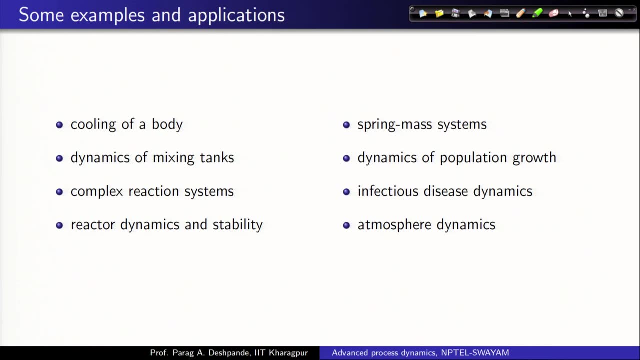 as well as non-linear systems in transform domain, and in either cases we will do continuous domain as well as discrete time domain analysis. This course would be inherently mathematical in nature, So every topic that we would start would start with a mathematical technique And followed by this mathematical technique. we will take an example from a process industry. 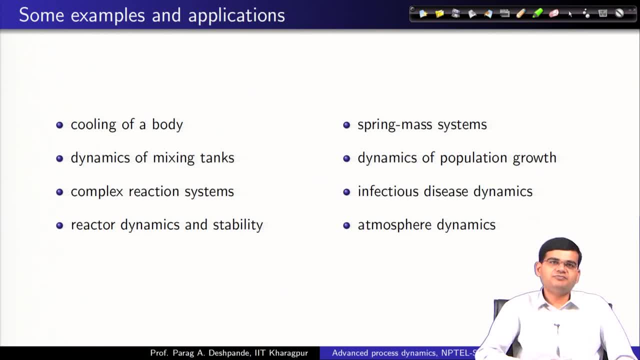 So what you can see here is representative examples. we will take much more of than what has been shown here, But on the left hand side you can see that we will typically take examples, for example, cooling of a body or dynamo, Dynamics of mixing tanks, complex reactions, kinetics or reaction dynamics and stability. 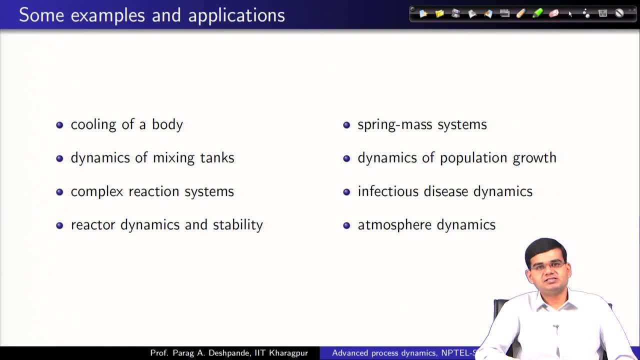 But, as I mentioned, the central premise of dynamical systems is the analysis of change. Now, changes take place in almost all domains of engineering as well as natural sciences, So therefore, dynamical systems would be of interest to mechanical engineers, aerospace engineers, biochemical and biotechnologists. 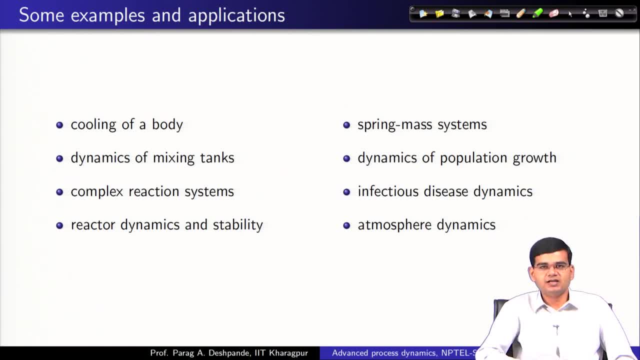 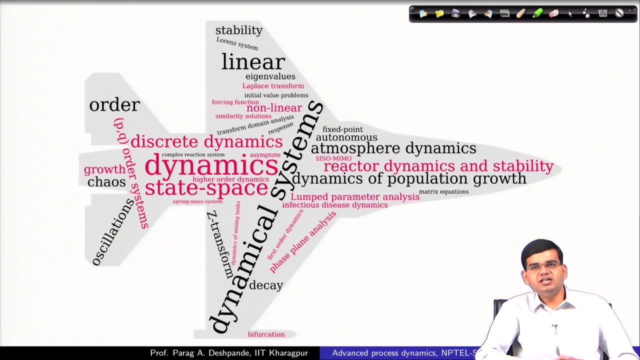 And fundamental physicists as well. So, therefore, we would be taking examples from other domains of science and engineering as well, making this entire analysis in the course truly multidisciplinary in nature. So I will leave you with this word cloud, which would give you an idea about every single.